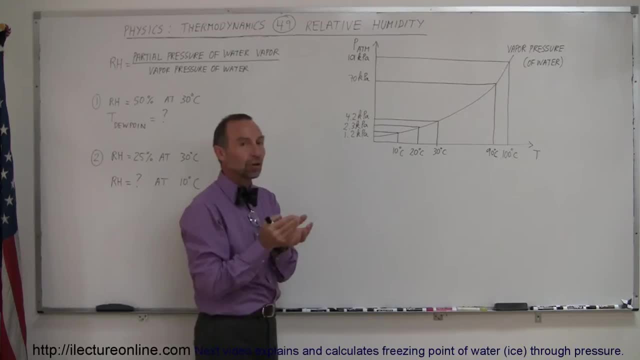 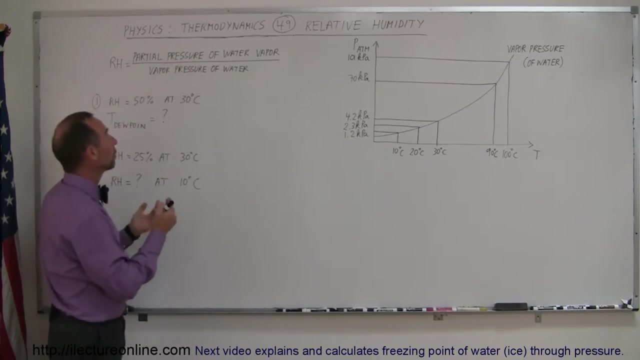 air can hold, and so the amount of pressure accounted for by the water vapor can go up. That doesn't mean it will go up. It means it can go up, and the relative humidity is the ratio of how much pressure actually is in the atmosphere accounted for by water compared to how much. 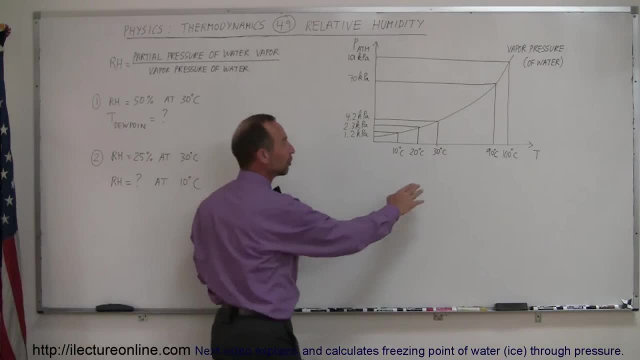 pressure water can actually be. For example, if the temperature is 30 degrees C, 4.2 kPa or the total atmospheric pressure of 101 kPa can be accounted for for by water. In other words, the water can be up to about 4.2% of the total pressure at 30 degrees. 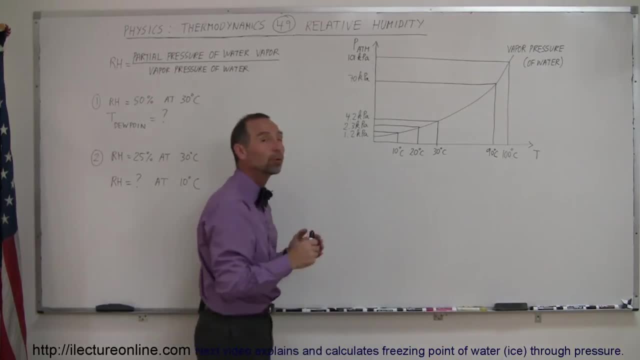 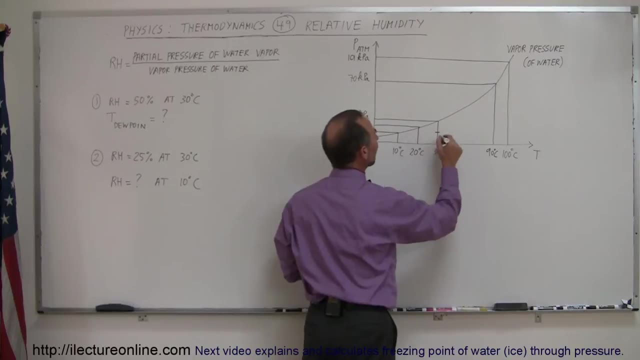 centigrade. At 20 degrees centigrade it can only be about 2.3% of the total pressure. So what that means is let's say that, for example, currently it is 30 degrees outside and the relative humidity 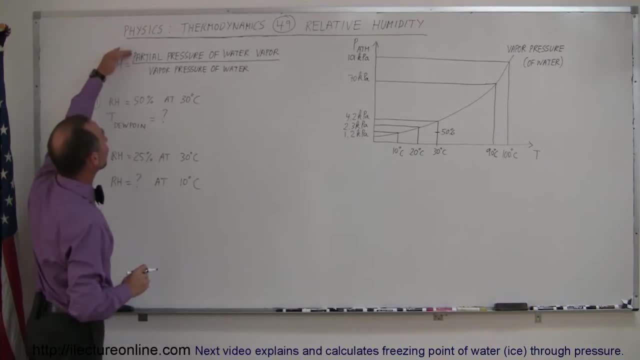 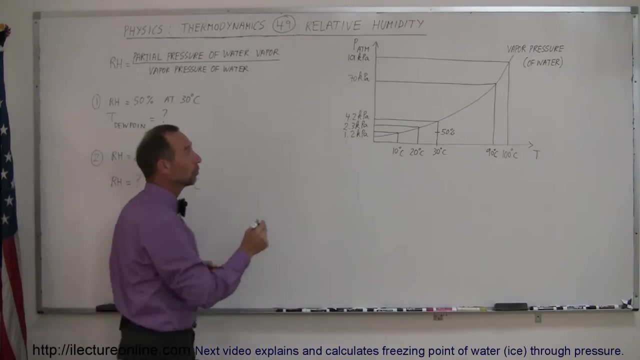 is 50%. What that means is that the ratio from partial pressure of water vapor to the vapor pressure of water is one half or one to two. What happens then when the temperature goes down? Well then, eventually you will hit the dew point. So if the temperature begins to cool, you can see. 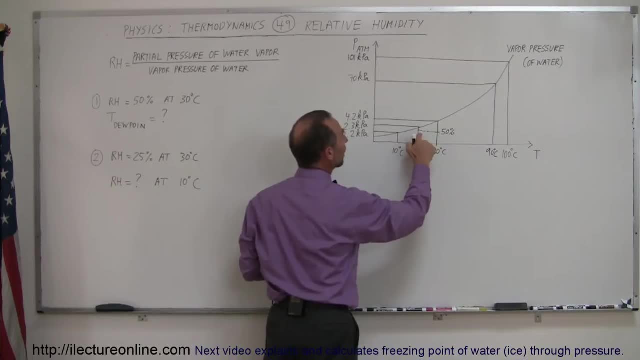 that, at 20 degrees centigrade, a much greater percent of what the atmosphere can hold is now water vapor, And then, if it continues to cool down, eventually you will reach what we call the dew point. In this particular case, as you can see, the dew point is at about. 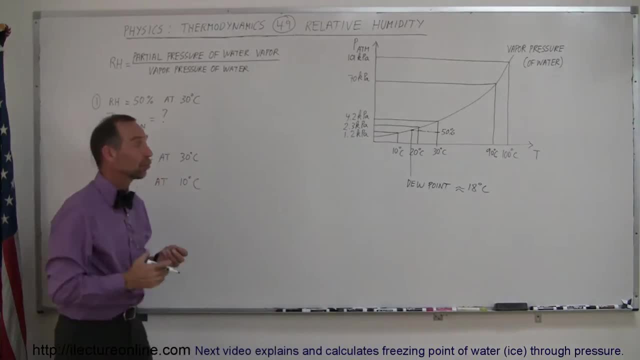 18 degrees centigrade, which means that if it's a warm day outside and it's 30 degrees centigrade, which is almost 90 degrees Fahrenheit, and it's 50% humidity, which is pretty humid for a hot temperature like that, as it begins to cool in the evening and the temperature drops below 18, 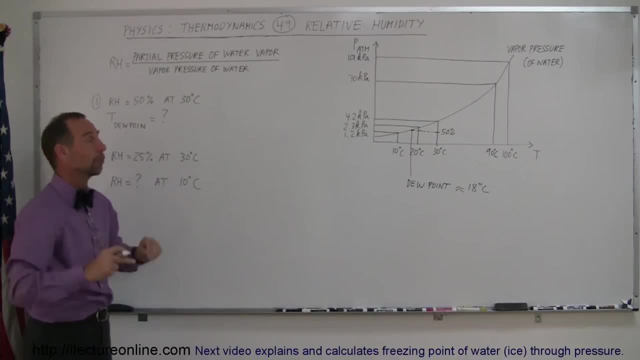 degrees centigrade moisture will become out of the air and you'll see dew forming everywhere on the surfaces around. As an example, let's say we have the relative humidity at 25%, which is not nearly as moist. So let's say we have the relative humidity at 25%, which is not nearly as moist. So 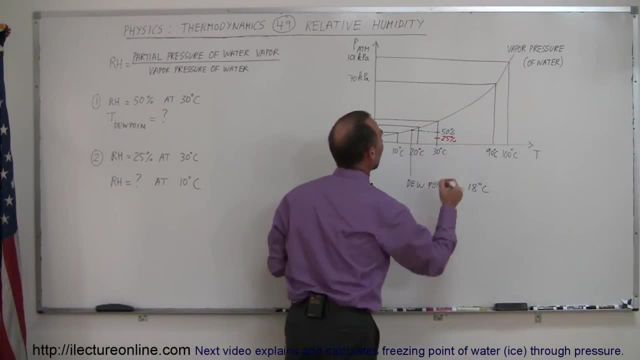 let's say we have the relative humidity at 25%, which is not nearly as moist. So let's say we have now come down here at 25% and let's say the air cools down until it reaches 10 degrees centigrade. 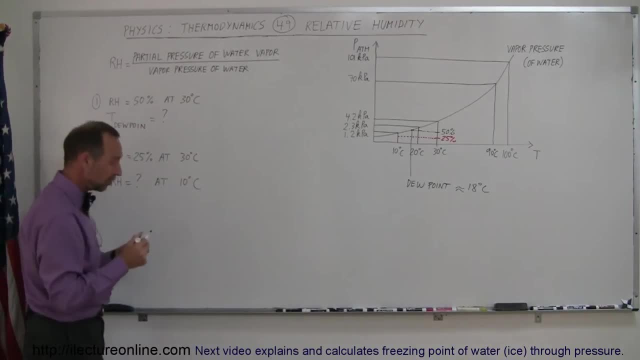 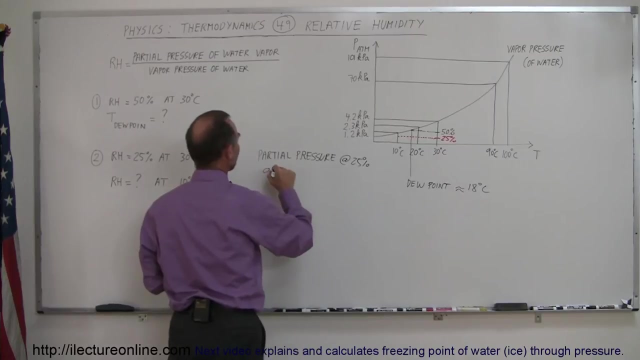 What will be the relative humidity at 10 degrees? if it was 25% at 30 degrees? Well, first of all, let's find out what the partial pressure is for water at 25%. So the partial pressure at 25% and 30. 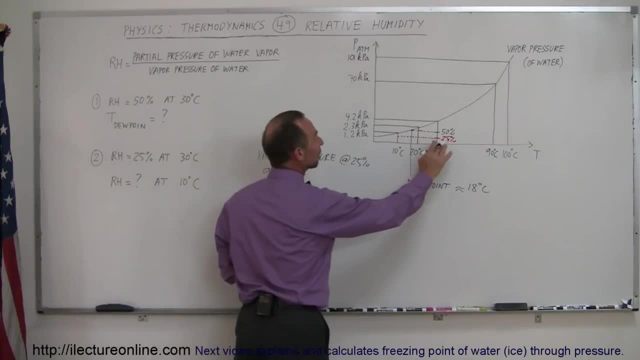 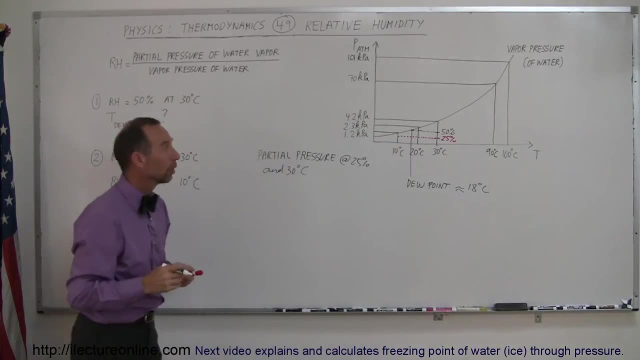 degrees centigrade is going to be 20 degrees centigrade, So let's say we have the relative humidity at 25% is going to be the ratio between what it can hold and what it actually holds. And so, since it can actually hold at 30 degrees centigrade, the atmosphere can hold a total of 4.2 kilopascals. 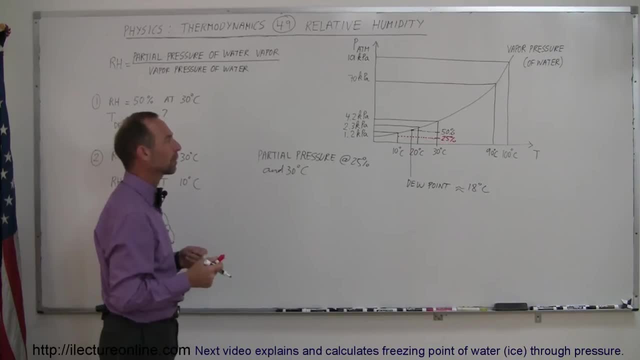 of water-vapor or the partial pressure of water vapor can be 4.2 kilopascals. If we take 25% of that, so 25% of the total that it can hold of 4.2 kilopascals is equal to 1, 0.05 kilopascals. 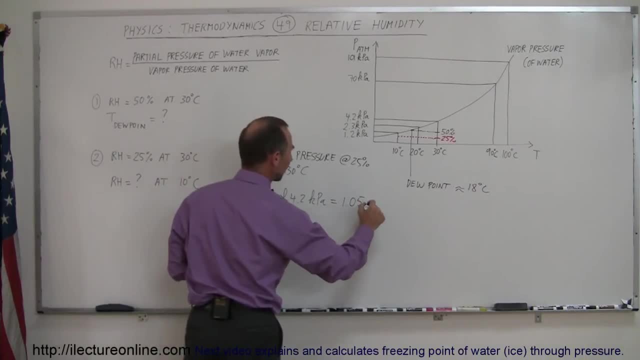 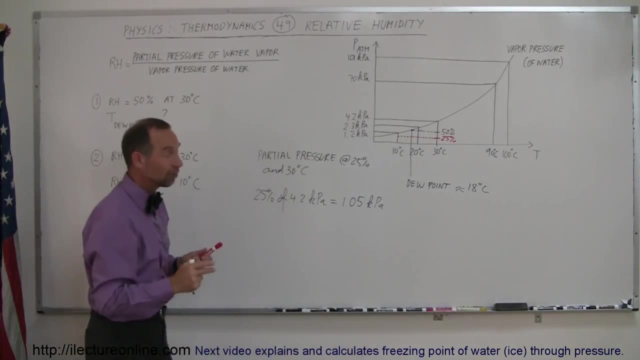 If we take 25% of that, so 25% of the total that it can hold of 4.2 kilopascals is equal to 1.05 kilopascals. So that means if the relative humidity is 25% and the temperature is 30 degrees, the 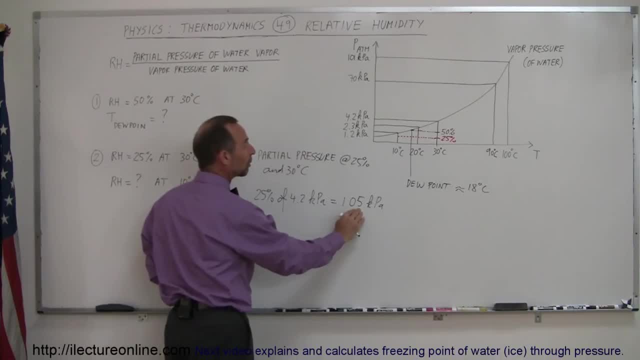 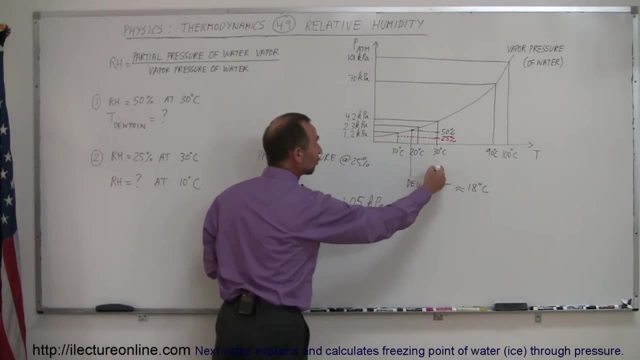 pressure associated with the water vapor in the atmosphere will be 1.05 kilopascals, which is about 1% of the total atmospheric pressure. Of course that doesn't change with the temperature cooling down, but now since at 10 degrees. 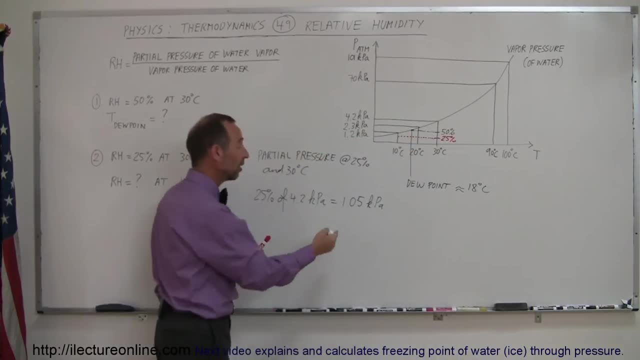 centigrade the atmosphere can only hold 1.2 kilopascals. 1.05 is almost as much as 1.2, so the relative humidity goes way up. So then the relative humidity at 10 degrees centigrade is equal to that ratio. the ratio. 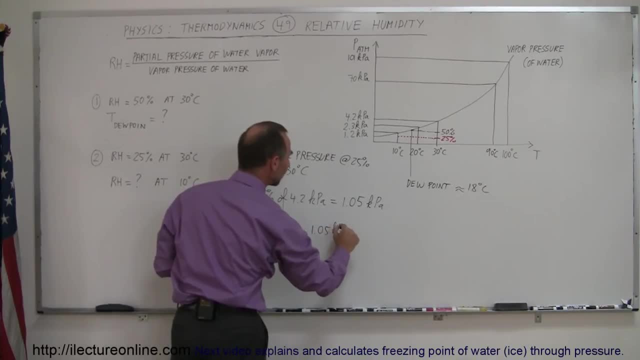 of what it actually is: 1.05 kilopascals divided by how much it can hold when it's fully saturated, which in this case is 1.2 kilopascals. And so, with my calculator, what is the ratio? 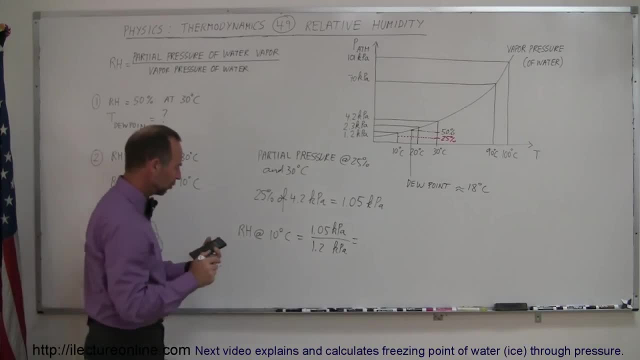 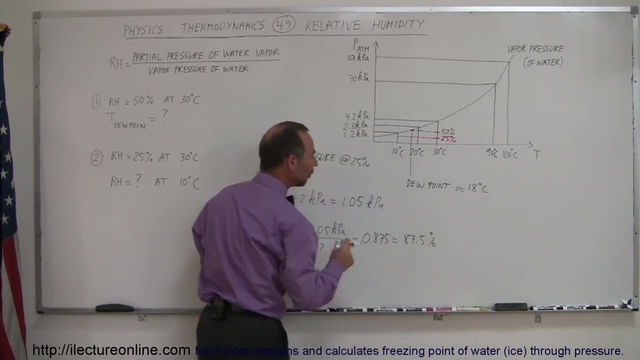 1.05 divided by 1.2, that is equal to 0.875.. Which is equal to 0.875.. So, again summarizing, that means that if the temperature was 30 degrees centigrade and the relative humidity was 25%, if then at night the temperature drops to 10 degrees, 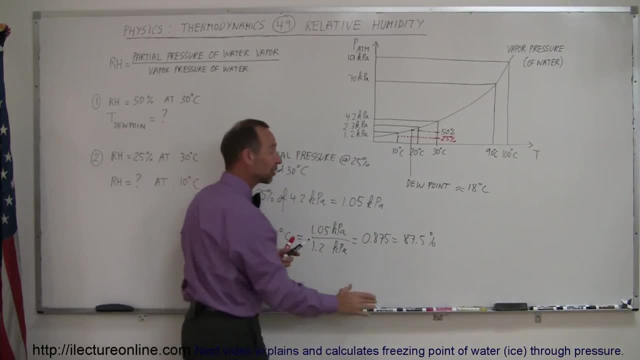 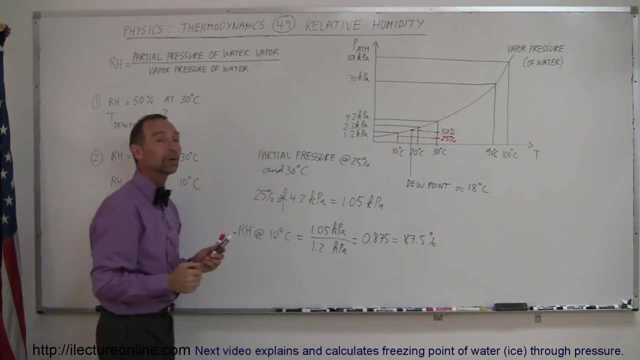 centigrade, the relative humidity with the same amount of moisture in the atmosphere will now be 87.5 degrees. You can see it doesn't have to cool down much more until we actually reach the dew point and moisture will become will start coming out of the atmosphere.